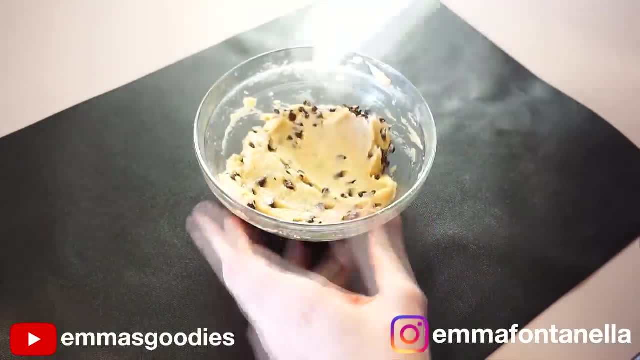 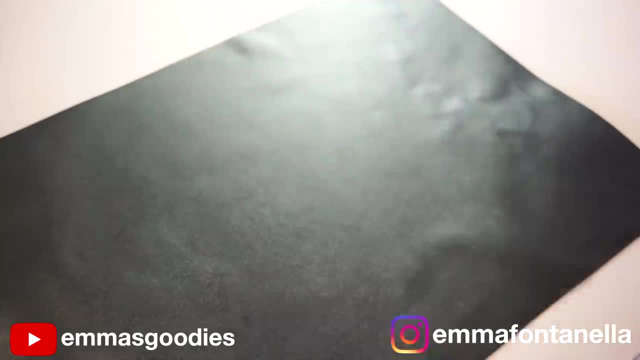 a little bit of sugar, if you want to add a little bit of sugar. if you want to add a little bit of sugar now. i personally love a good, fresh, creamy cookie dough. just look at that. it's delicious. however, i needed a thumbnail, so i'm gonna pop this in the fridge. that way i can get some pretty scoops. 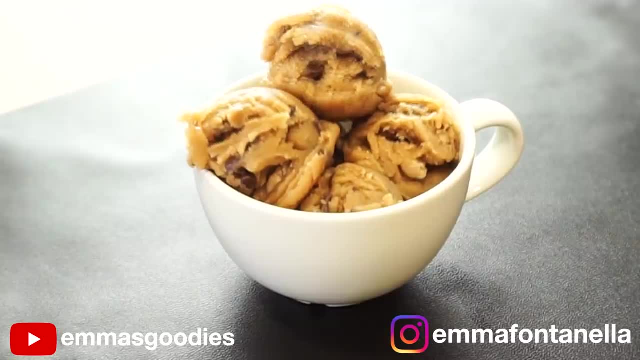 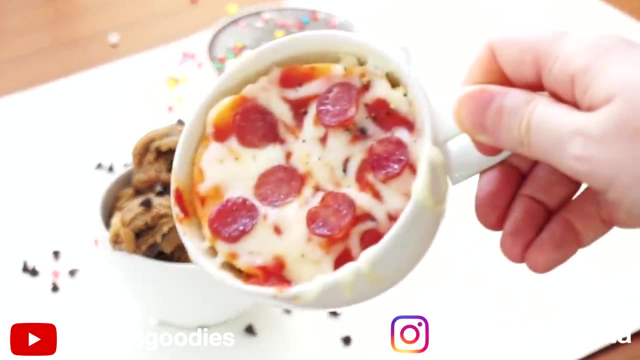 if you love cookie dough, you will scream of joy when you try this. it's sweet and salty, so simple, but so amazing. have it as is. top your ice cream with it. it's delicious. moving on, we're gonna make stuffed crisp pizza in a mug, perfect for any time you want a quick savory snack now when i say pizza. 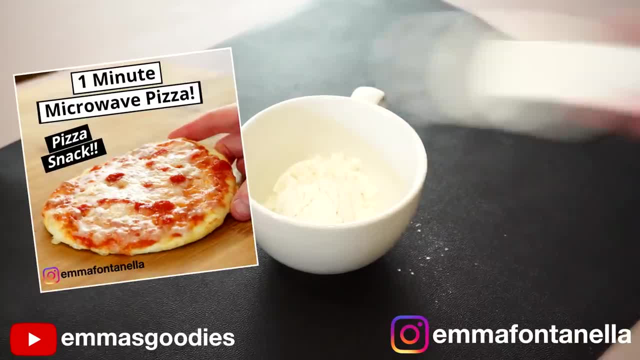 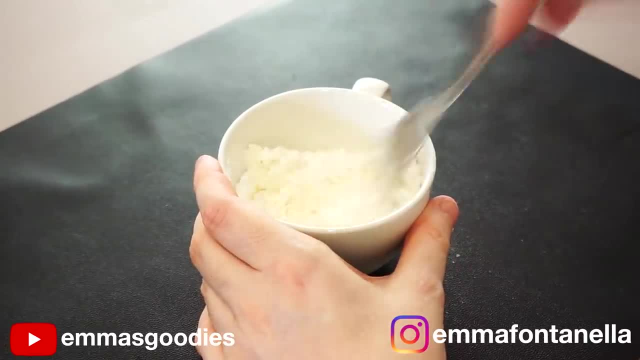 i mean pizza pizza. if you want an excellent, delicious microwave pizza, i have made it link in the description box. it's just as amazing as mug pizza. hell, no, it's better. okay, i get it, though sometimes you just want a quick savory snack in a mug combined flour, baking powder and salt. give. 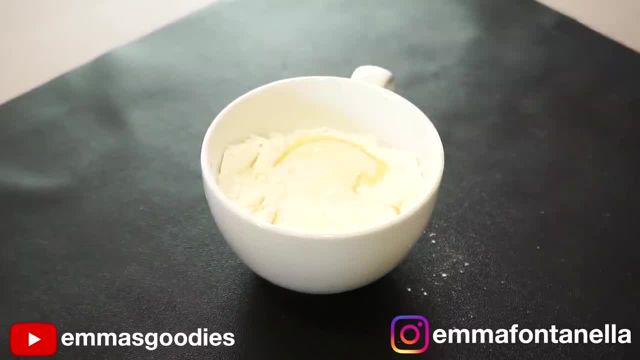 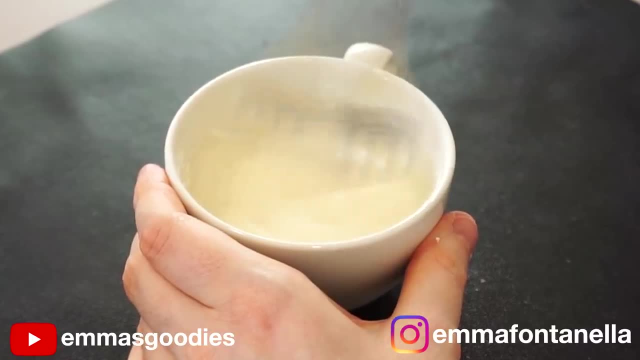 everything a rough toss and add the oil and milk. now, when i was developing this recipe, i was quite disappointed because once you've eaten that top cheesy crust, you're left with the sad crumb. the cheese to crumb ratio is just not good. so we're making the top cheesy crust and we're going to make the top cheesy crust. 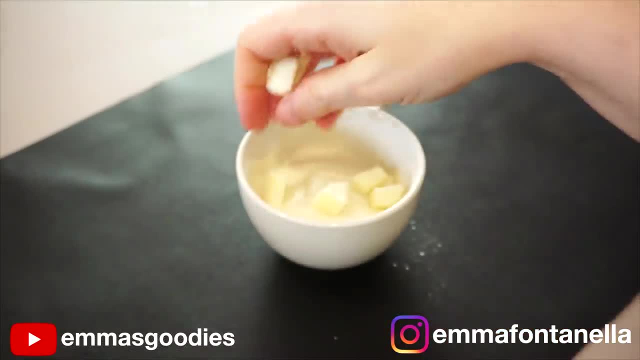 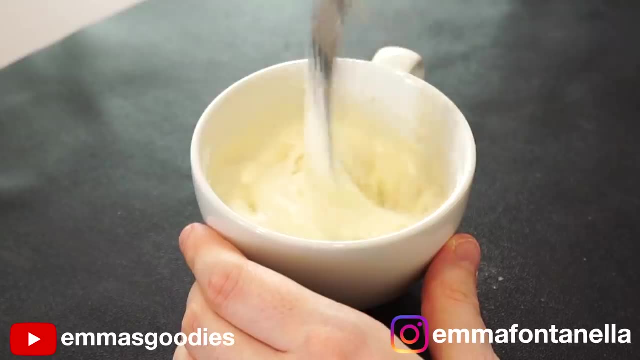 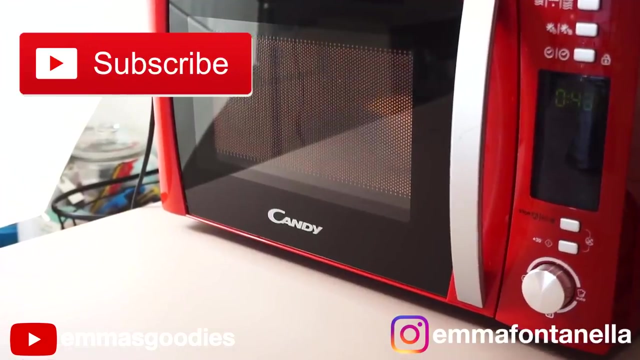 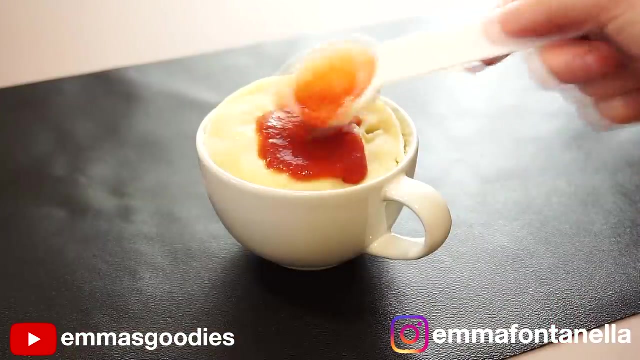 and i will tell you how to make it. i'm gonna look it up and i'm gonna give you a little bit of a test. first, check out the video. you'll get the audio here in a moment, but this video is more about making stuffed crust pizza. get yourself some cheese- the more flavorful the better- and add that to your batter. we're going to part-mix the crust. that way the cheese starts to melt and become all gooey and delicious. so microwave your mug pizza on high for about 45 seconds to one minute. if you're new to my channel, hello there, welcome. make sure to subscribe and click that bell. i post new videos every week. add the pizza sauce, any seasoning you like- the more the better- the cheese and any other toppings you like. i had pepperoni, but no, i would give it a thumbs up and i hope you enjoyed this video a lot and i'll see you in the next one. 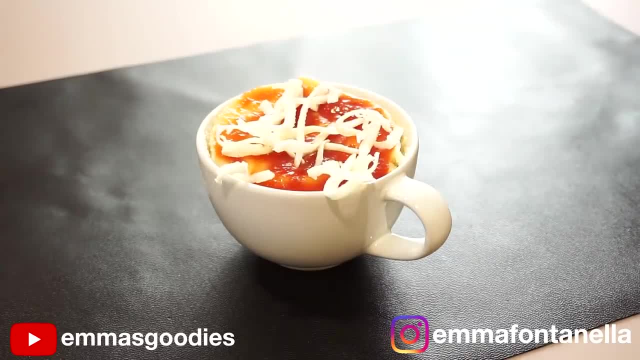 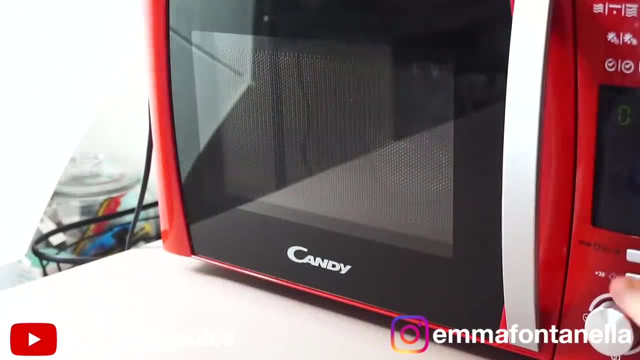 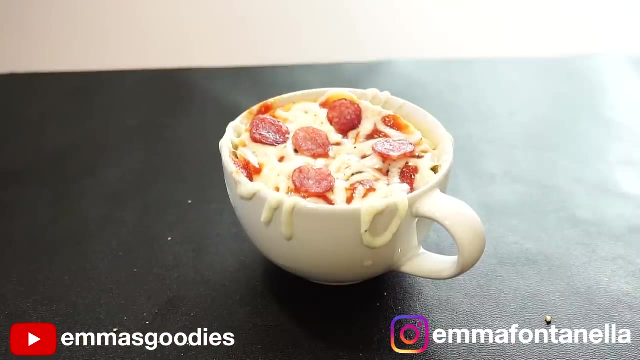 bye cheese and any other toppings you like. i had pepperoni and i forgot to add it, so don't mind me adding it at the end. pop this baby in the microwave just for about 30 to 45 seconds. we just want that cheese to melt. add the pepperoni if you forgot it, and you got right there the most. 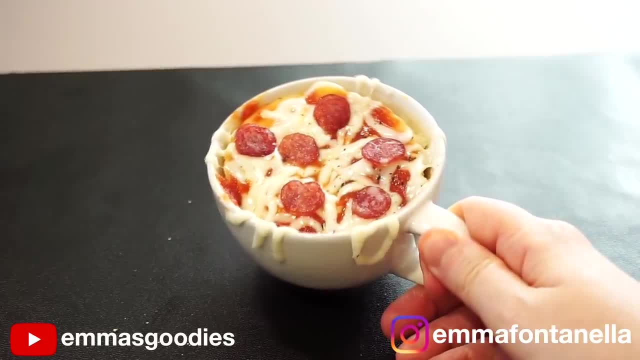 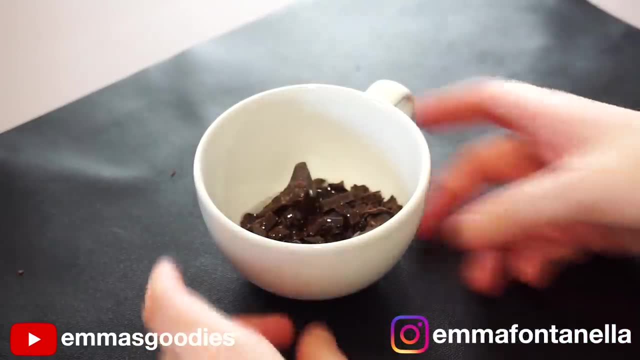 delicious domino stuffed crust pepperoni pizza in a mug. i've saved the best for last. this is my favorite, and that's cosmic brownie in a mug. into the mug goes the chocolate chopped into small pieces and some butter. you want to pop this in the microwave, stirring it every 30 seconds until.